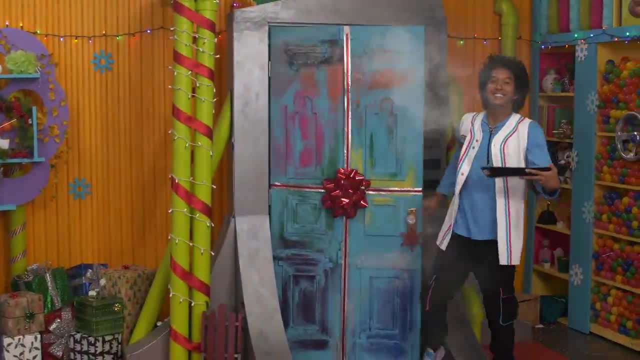 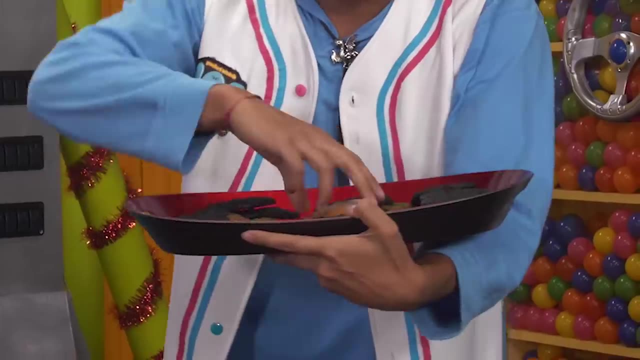 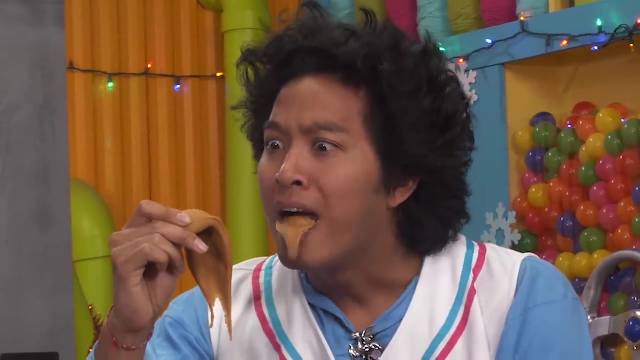 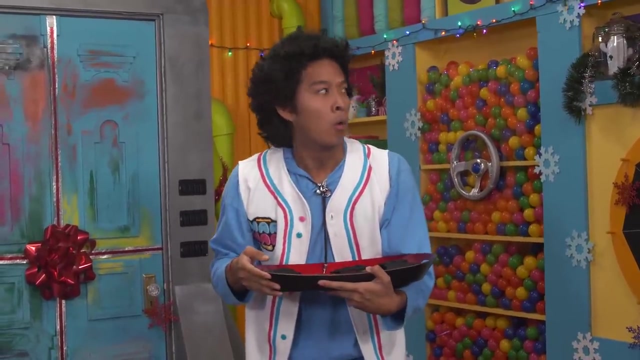 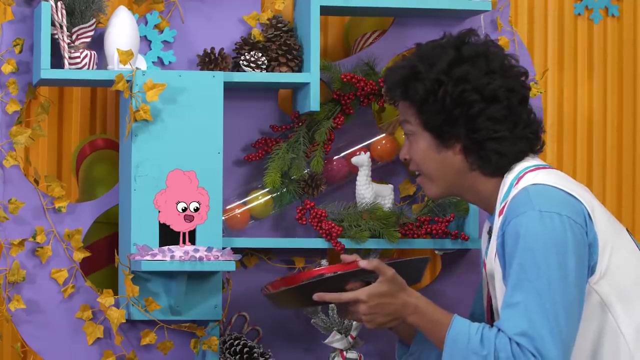 Surprise, Delicious cookies. Huh, where's everybody? I guess I could sneak one before anyone gets here. That is not right. Did someone say cookie? Oh hey, Cloudy, Do you want to try one? Marmar, did you mix up your cookie recipe with your gummy recipe? 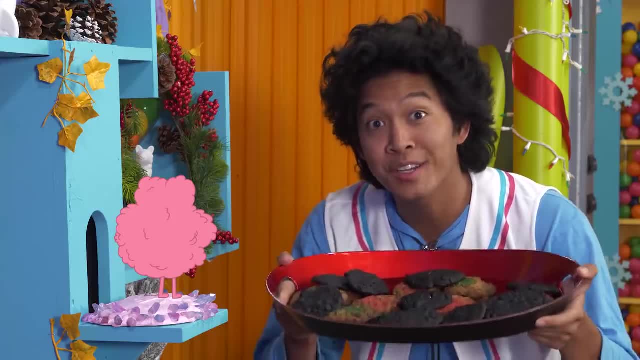 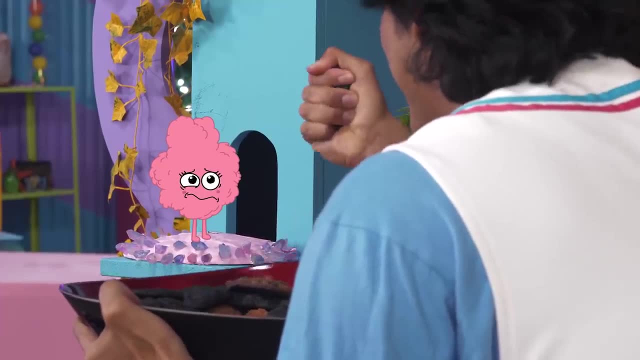 Cloudy, these cookies are great Explorers. do you want to try a cookie? I bet yours will be perfect. You don't even want to try one. Okay, maybe my cookies didn't turn out exactly how I wanted them to. 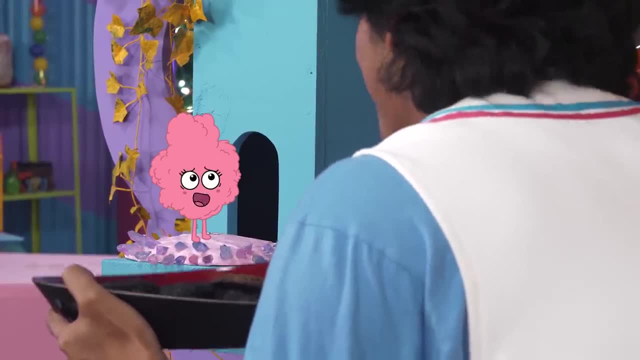 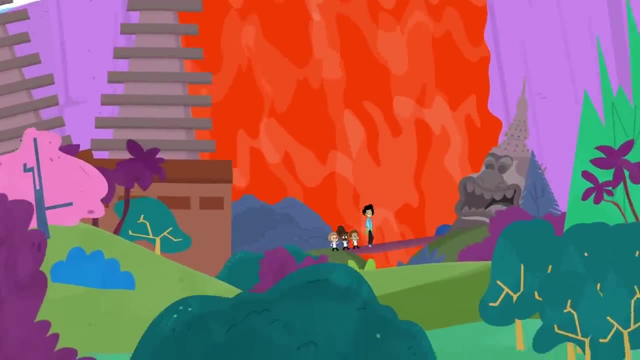 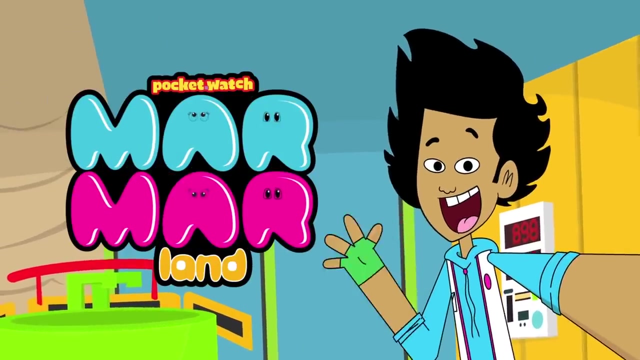 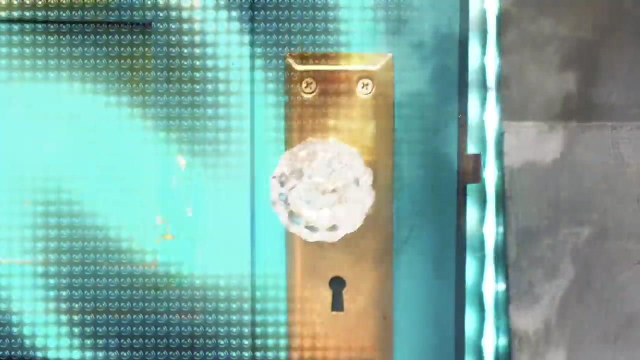 You might need a little help baking Marmar. I think you're right and I know exactly who can help me bake the perfect batch of cookies. Here's the magic door it's time to explore in: Marmar, Hi Marmar. 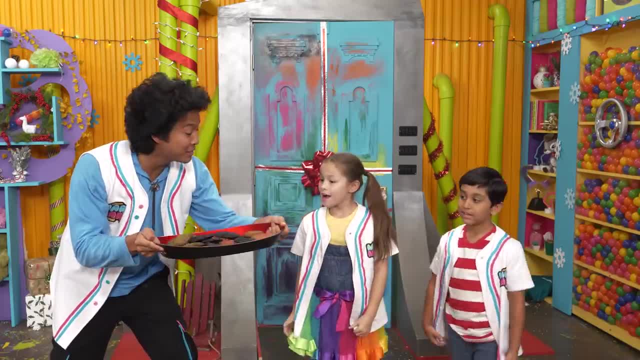 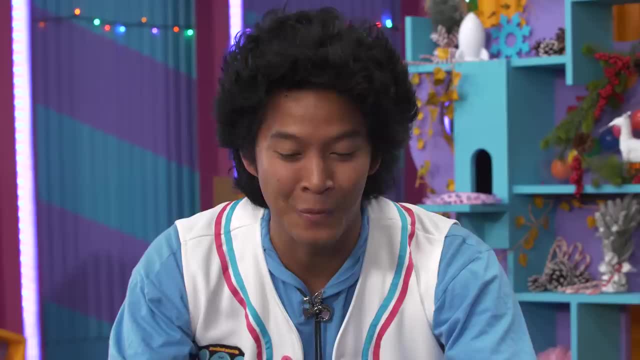 Hi Hayden, hi Ayush, Just in time, I wanted to surprise you guys with some holiday cookies, but they didn't turn out so right, So I figured we can bake some new ones together. Let's do it To the lab. 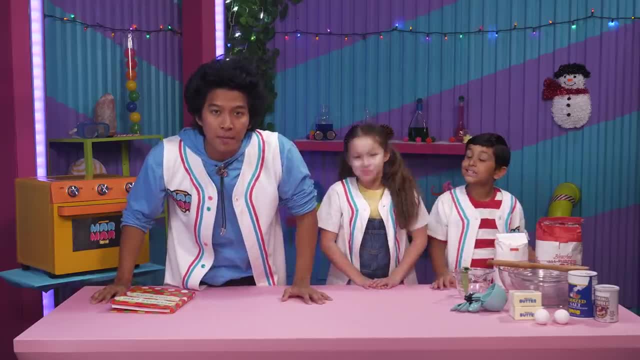 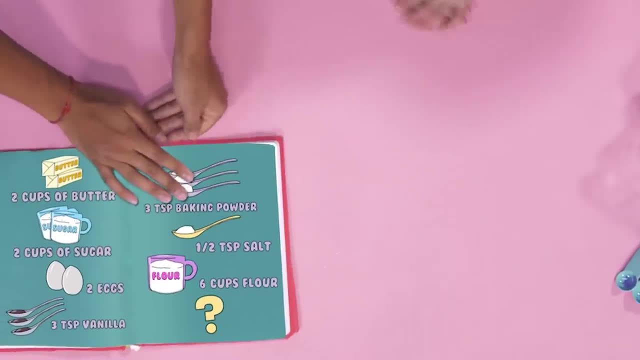 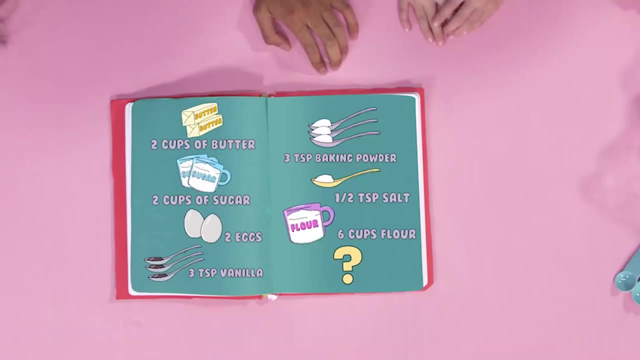 We washed our hands, so let's go. Explorers, always remember to wash your hands before cooking or baking, to keep things safe and germ-free. Oh no, We're missing an ingredient. Cloudy Cloudy, it's okay. 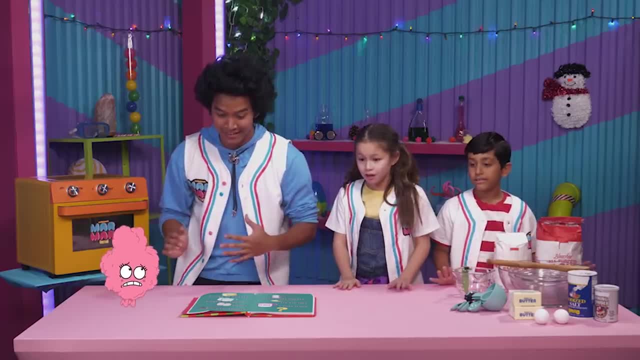 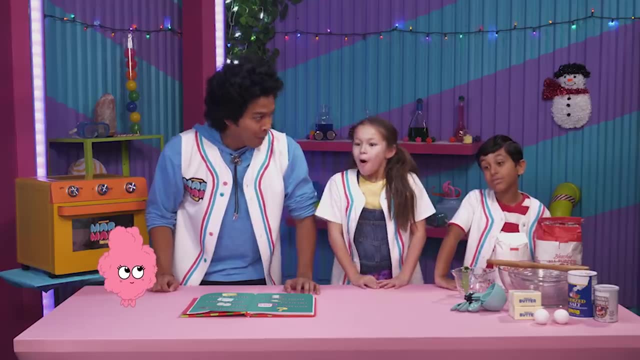 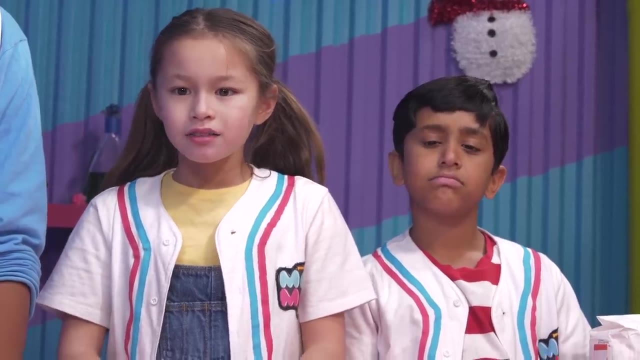 We're missing an ingredient. Stay calm, I have an idea. How about you go get the missing ingredient while we start the recipe? I'll keep the ingredient a surprise. I love surprises. Cloudy, can you give us a hint? Here it is, You don't need the surprise ingredient until the very end of the recipe. 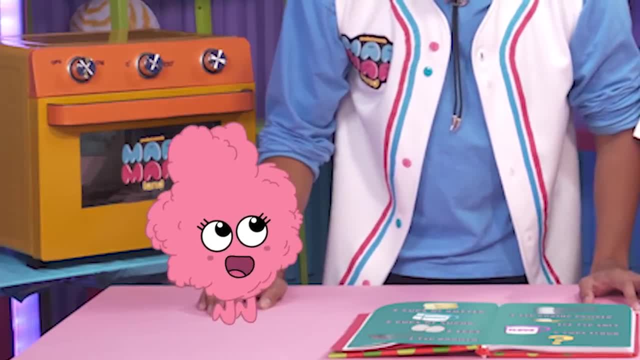 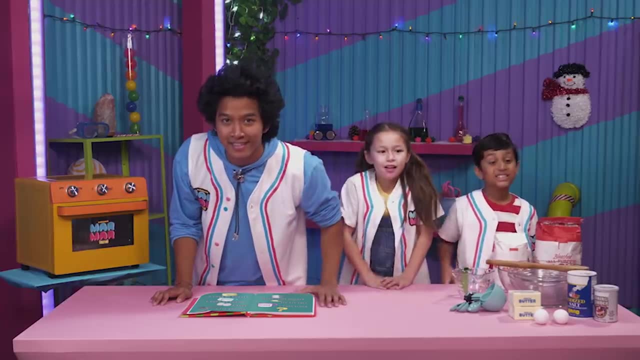 Can anyone guess what the surprise ingredient is? Elephant, boogers, Chinchilla hugs, All interesting ideas, Explorers. what do you guys think it is? All good guesses, But think hard, Because I'm going to make this a challenge. 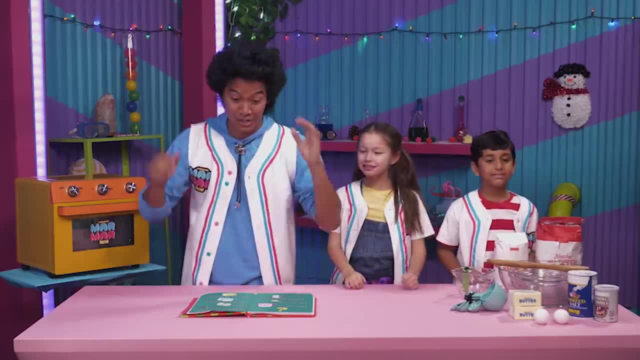 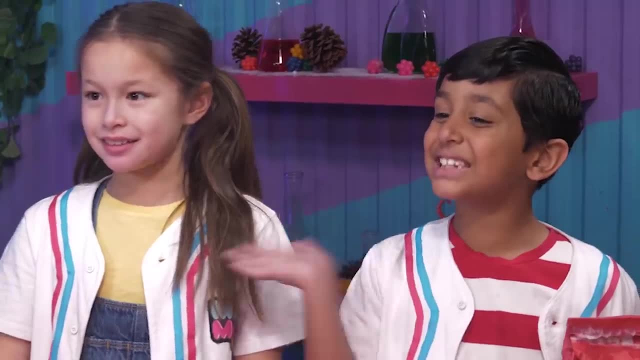 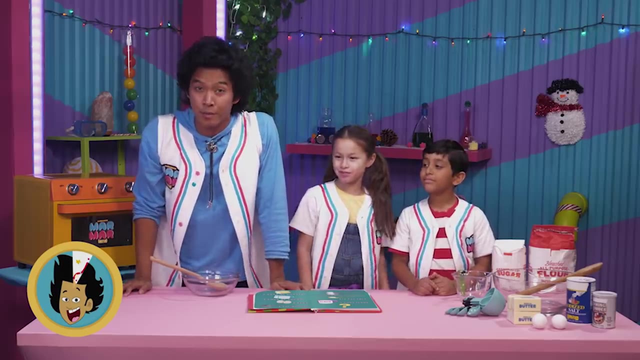 Yay, Okay, we have to finish the cookies before Cloudy gets back with the missing ingredient and the Mar-Mar timer goes off. We better get started. Thanks, Cloudy, See you soon. Okay, Explorers, the first step is to preheat the oven to 350 degrees, so the oven will be ready right when the cookie dough is. 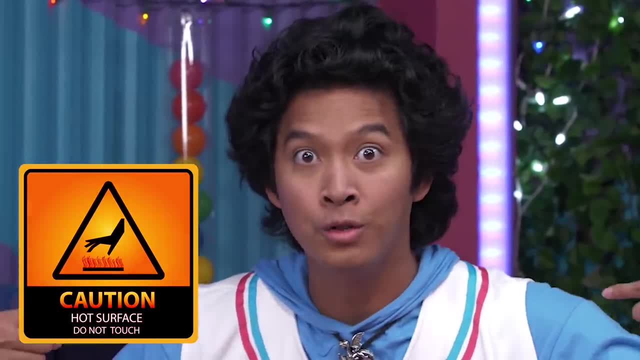 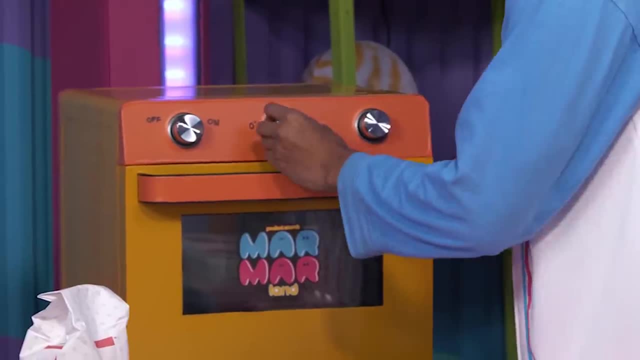 Explorers, do not touch the oven. Make sure you have someone older and responsible who can help you in the kitchen with stuff like that. Safety first, I'll handle this part. Done, Okay. the next step is to add butter and sugar. 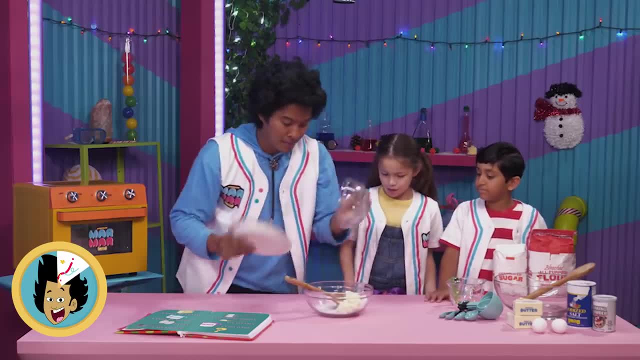 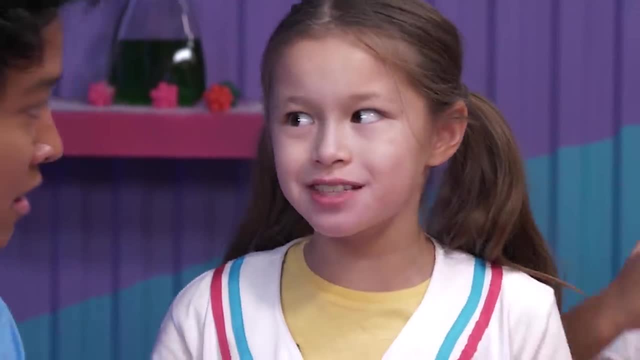 Hmm, sounds easy enough. Butter, Bang, bang And uh-huh, Here we go. Yeah, like that, Whoa, whoa, whoa. Hold on, Mar-Mar, We have to measure them first. Oh, how silly of me. 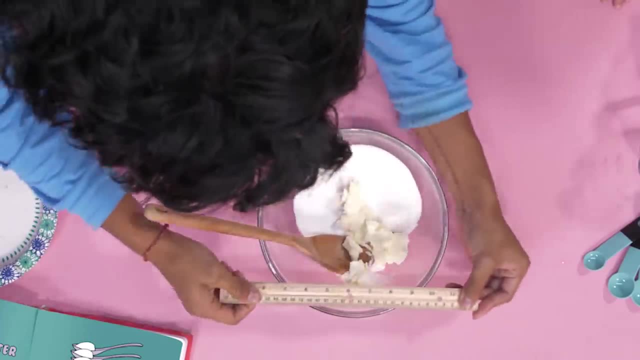 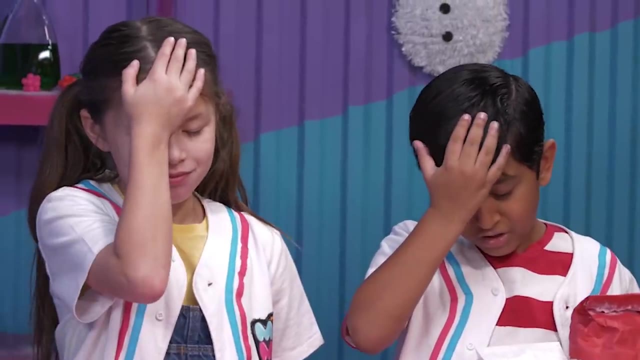 Measurements, Measuring, Here we go. That's the wrong kind of measuring, Mar-Mar. Oh, that's what I did wrong before. Oh, brother, Um, okay. I'll read the ingredients and measurements out loud so we know we have everything before we get started. 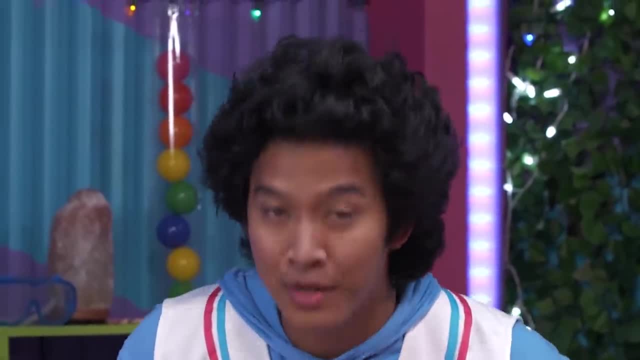 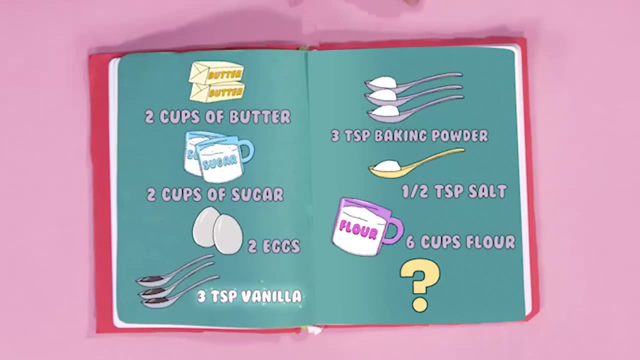 Remember Cloudy is getting the missing surprise ingredient, but we won't need that until the very end, So we're gonna need two cups of cubed butter, two cups of sugar, two eggs, three teaspoons of vanilla, three teaspoons of baking powder, one half teaspoon of salt and six cups of flour. 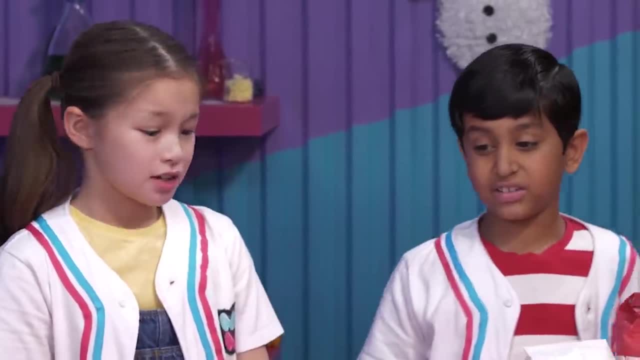 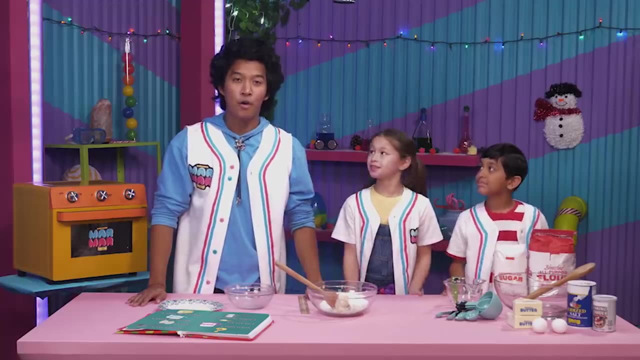 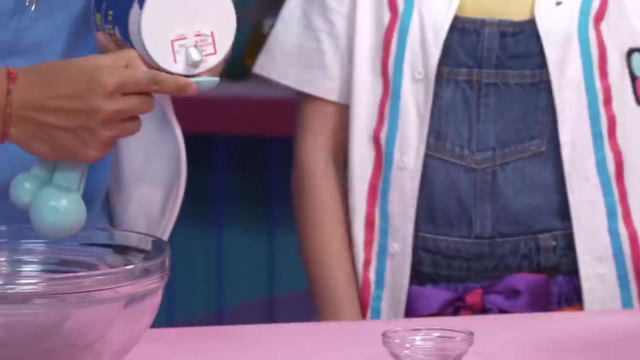 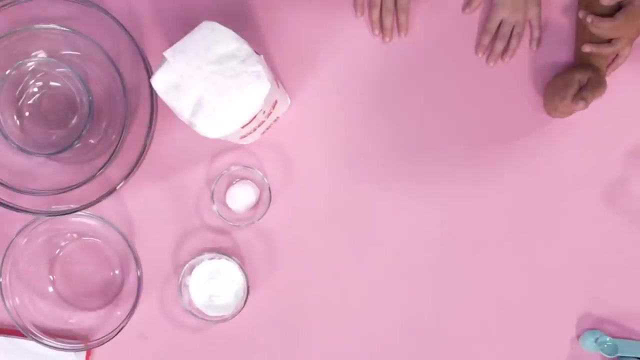 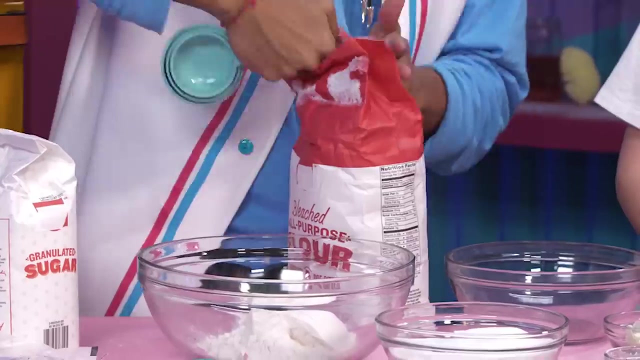 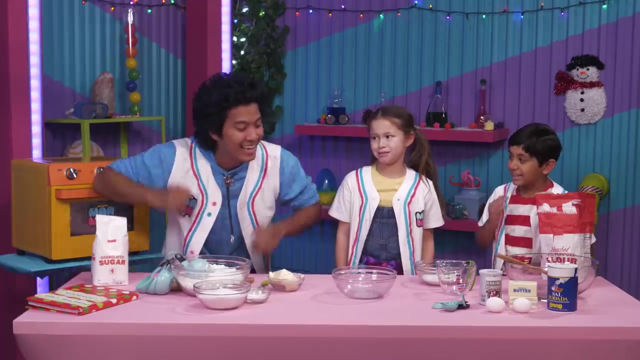 That's a lot of ingredients. Mar-Mar, can you please help us? Sure thing, Explorers, never be afraid to ask for help. This calls for Marlin and Mar-Mar Mise en place. Catch your breath, Mar-Mar. You aren't making any sense. 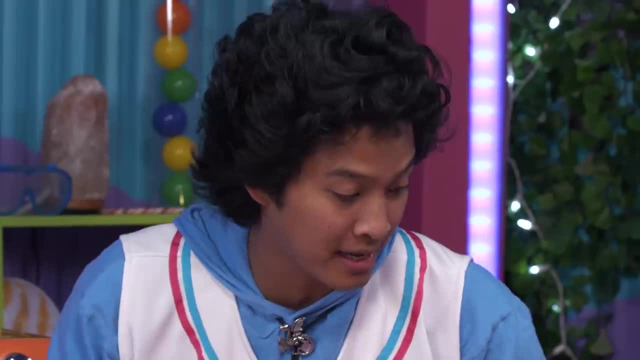 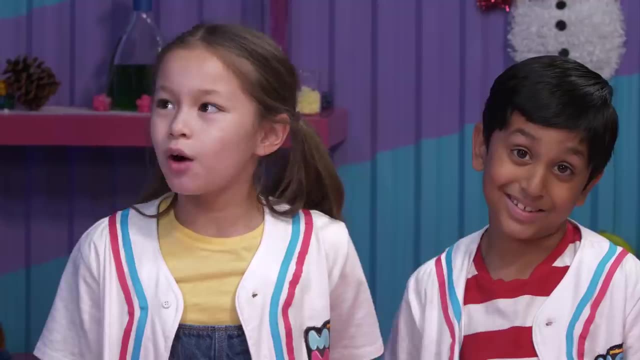 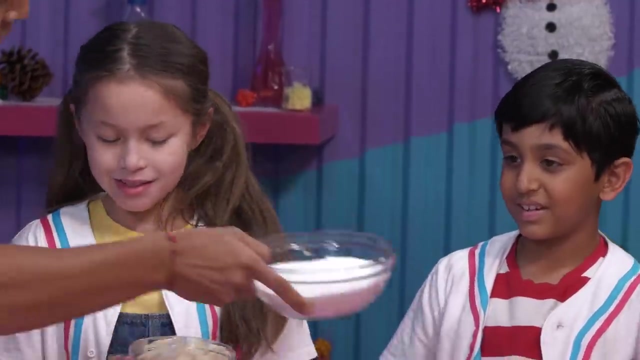 No, mise en place is French, It means everything in its place. The more more you, Mar-Mar, Mise en place. So let's bake. What does the recipe say? we add first Two cups of sugar. two cups of butter. Hayden, you pour in the butter, Ayush, you pour in the sugar, And then you both can take turns stirring. 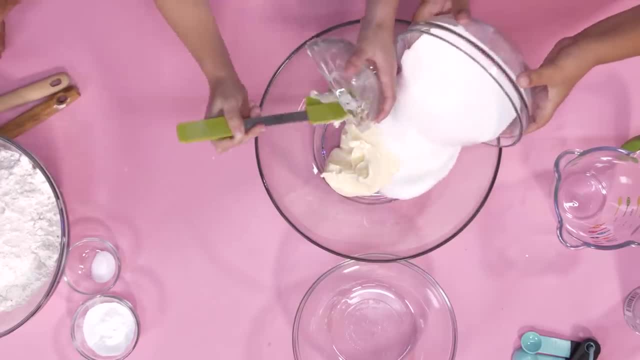 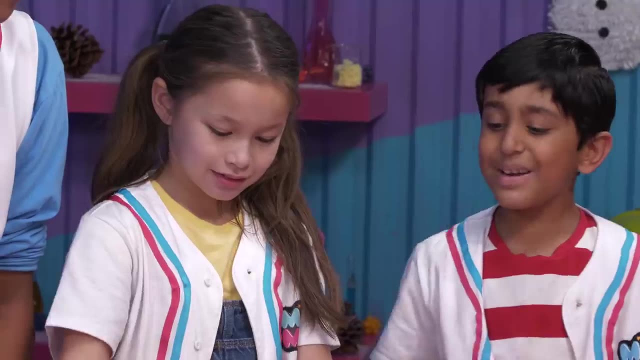 Thanks, Nice, Let's do it. Whoa, Whoa, It's sticking. Whoa, Whoa. Teamwork makes the dream work. All right, next up two eggs. I got this, guys, One and two. 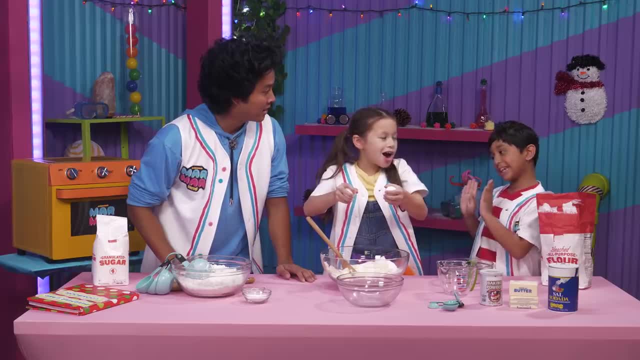 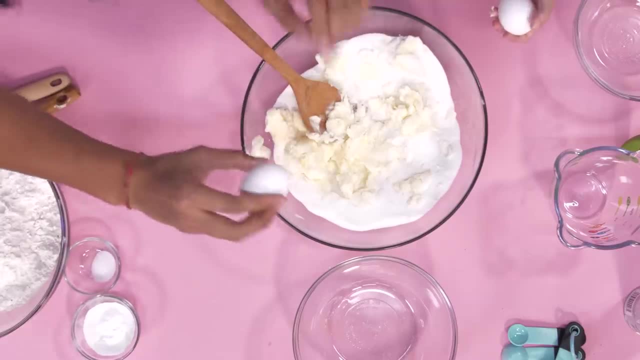 Wait, Hayden, You're supposed to crack the eggs first. Oh Yeah, gently crack the eggs on the corner of a bowl, just like this, and then put them in there and try not to get any shells in there. Okay, Oh gosh. 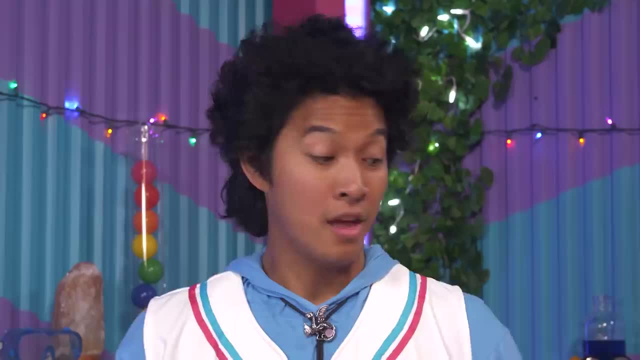 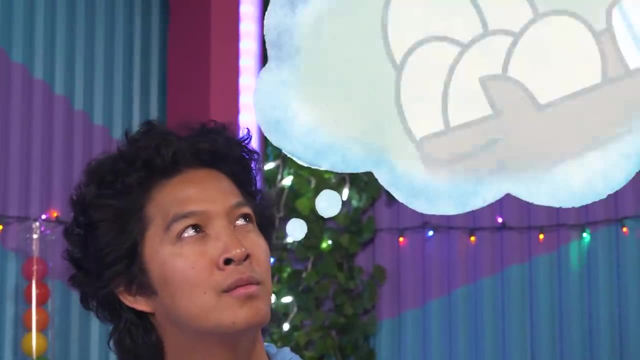 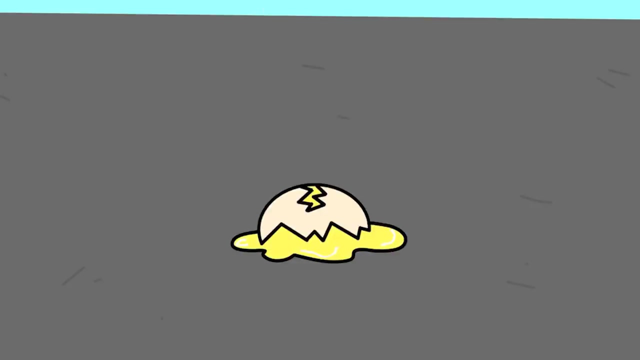 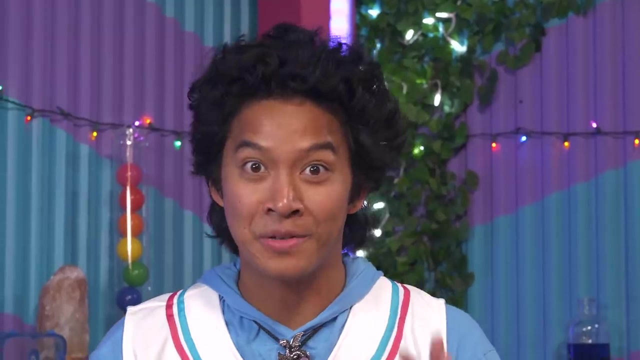 That's good, That's good. Okay, Yeah, Great job, Explorers. Hmm, I wonder what other ways are there to crack an egg? Wow, Those are some pretty crazy ways to crack an egg, but they only work in cartoons. 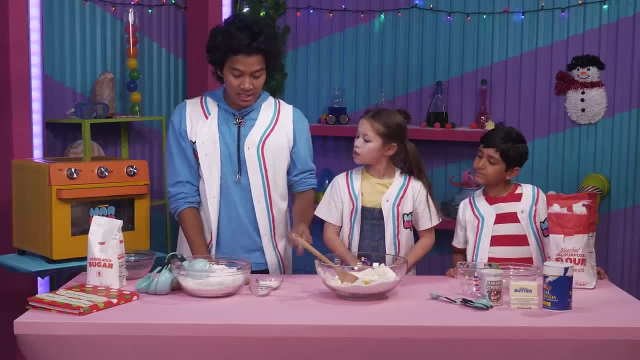 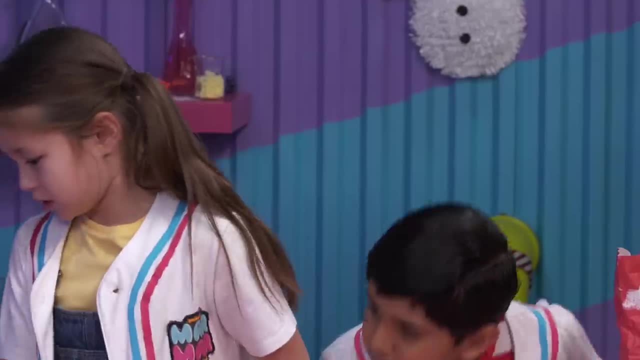 Back to the surprise cookies. Yes, Okay, We're going to need three teaspoons of vanilla and three teaspoons of baking powder. Murmur, where'd you put the vanilla? Oh, Uh, No, That's not it. Whoa Yeah. 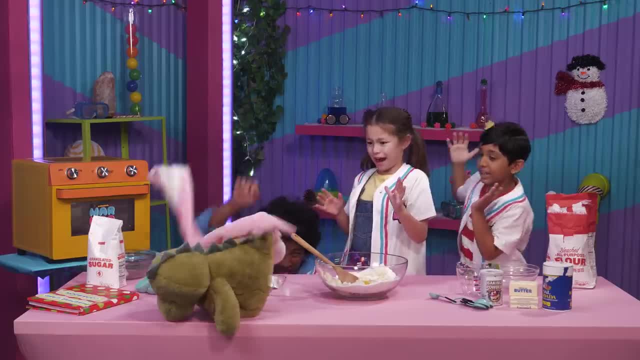 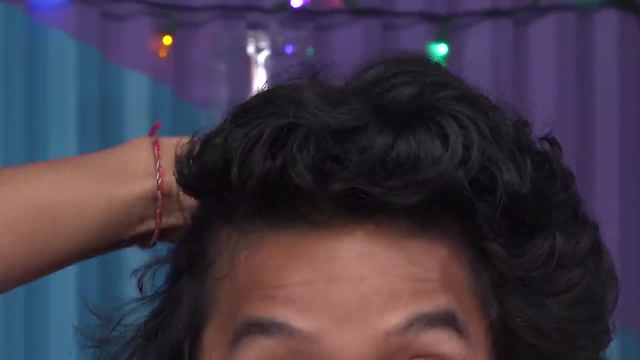 Whoa, Is that a track? Ah, Whoa, Whoa, Oh. no, It's a shark. It's a shark, I know Let's go to the hair. Oh, Ow, Ow, Oh. Is that a track? 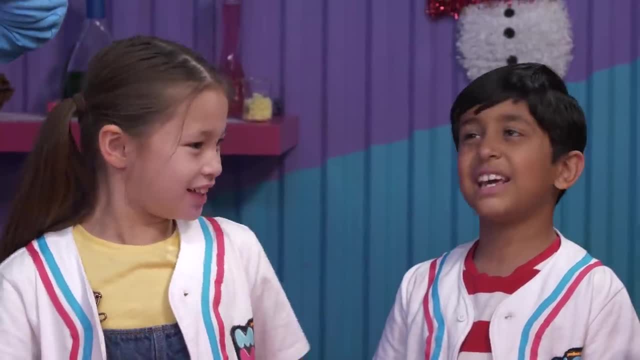 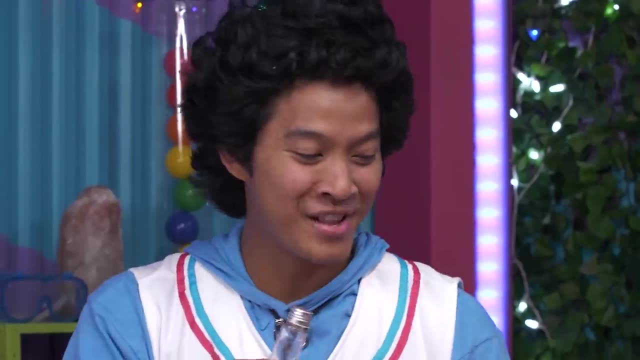 Is that? Is that like an elephant? Is that an elephant? Is that an elephant? Is that an elephant? Oh, Oh, Here it is. Whoa, All measured and ready. Mm, Let's pour it in Whoa. 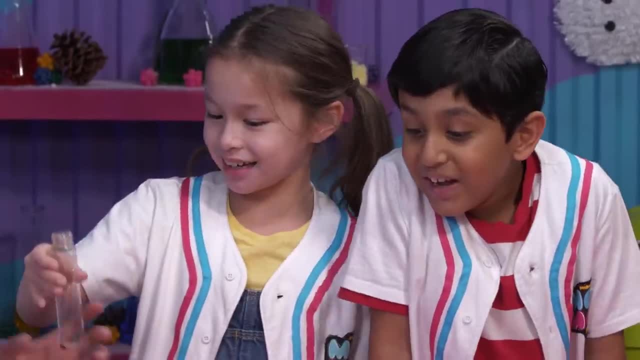 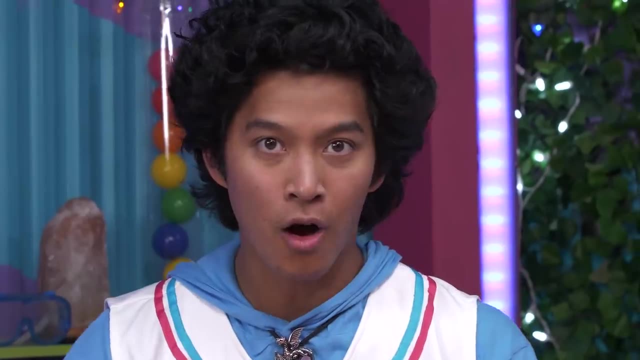 Whoa, Here it goes. Okay, Here you go. Now let's add the baking powder. Yeah, Let's do it. Woo Woo, Woo Woo. We are racing through this recipe, which is a good thing, because the Murmur timer is. 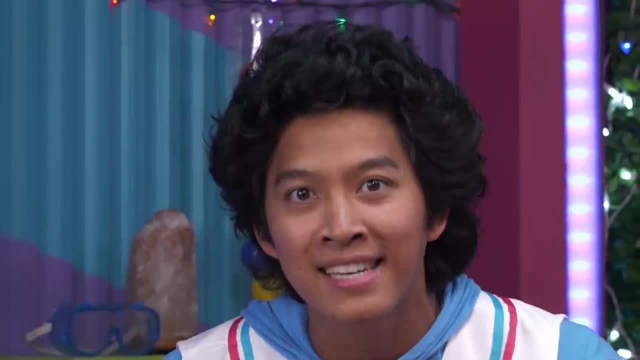 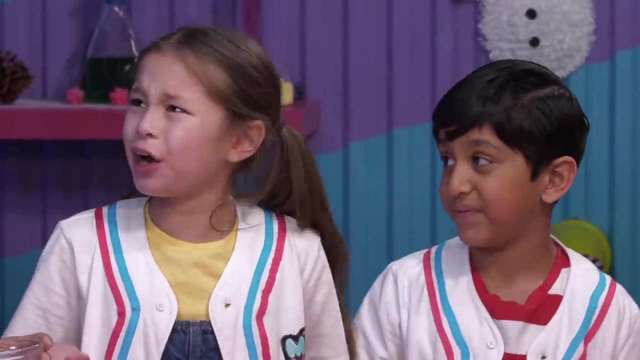 almost up, which means Cloudy is almost back with the surprise ingredient. What's next Murmur: Half a teaspoon of salt. Why are we adding this to cookies? Salt actually balances the sweetness and it makes cookies so much better, I promise. 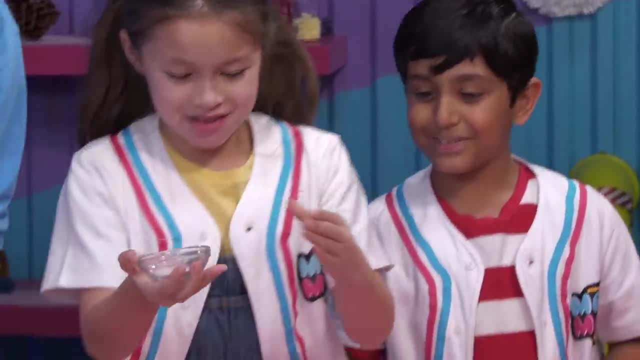 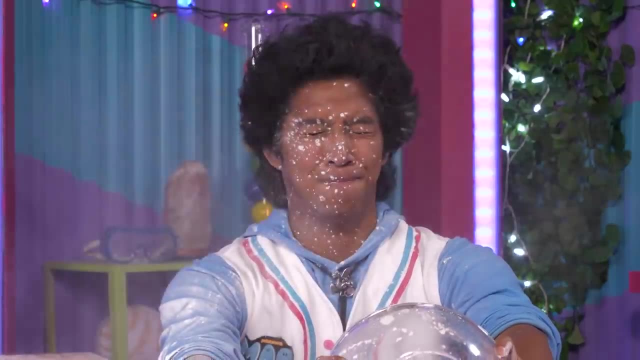 Go ahead, Put it in, Sure, I guess. Okay, Wow, Last step: six cups of flour. Okay, Okay, Murmur, You look like a ghost, Do I? Maybe we should add the rest of the flour, Okay. 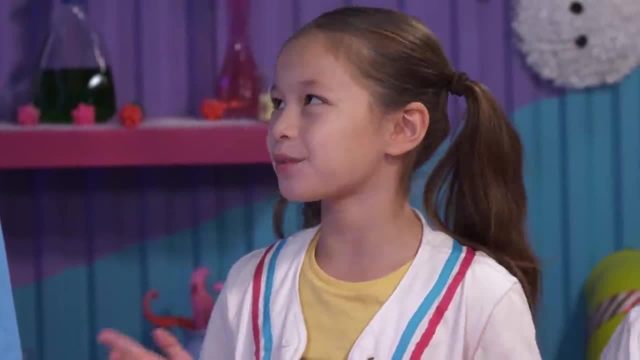 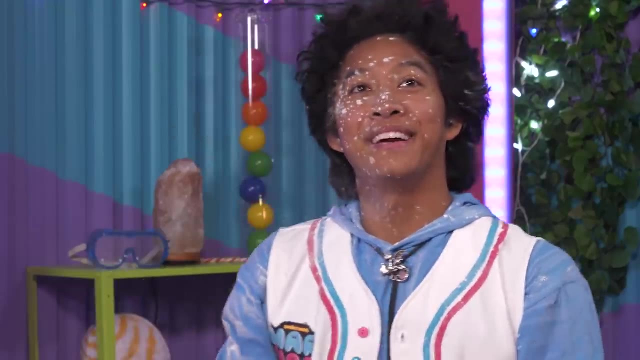 Okay, Okay, Okay, Maybe we should add the rest of the flour a little more carefully. Murmur, Yeah, I agree with Hayden. Can I get a little help here? Ah, Much better, Thank you. There we go, Nice. 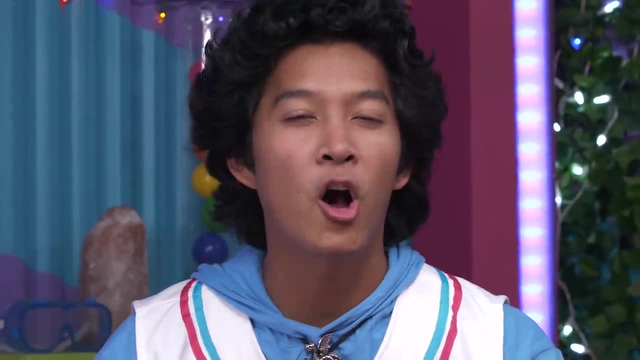 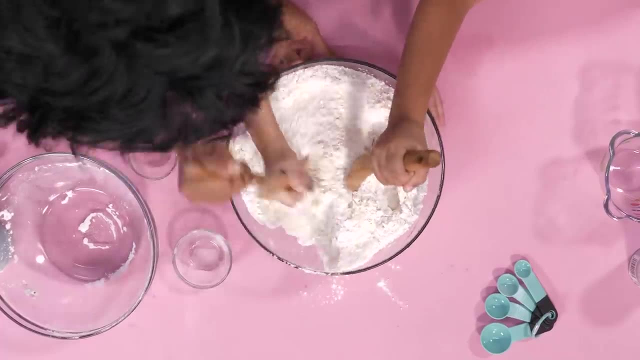 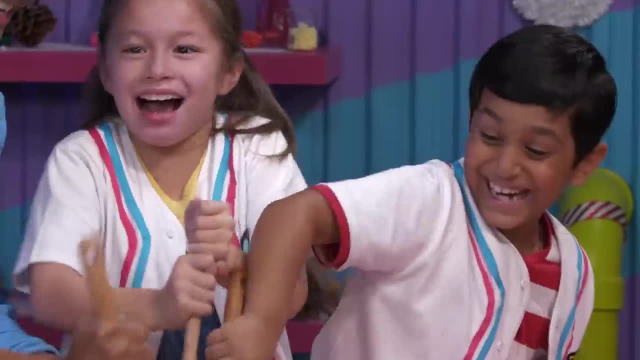 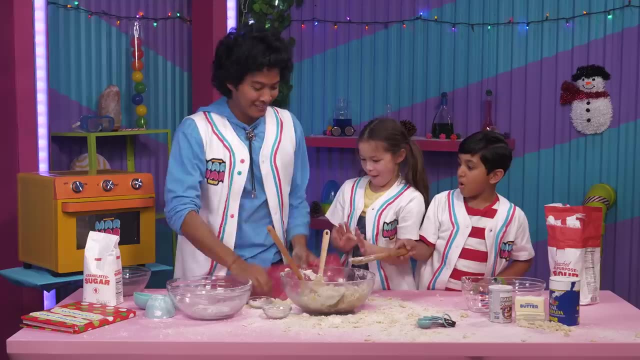 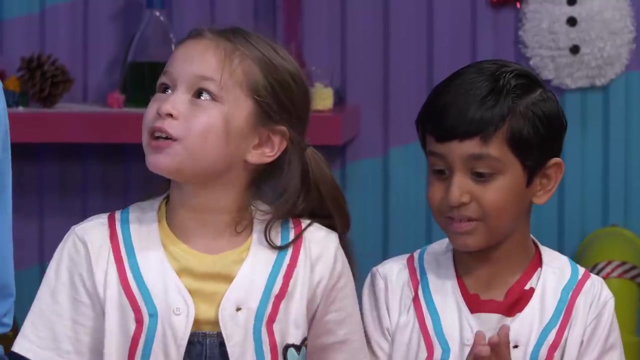 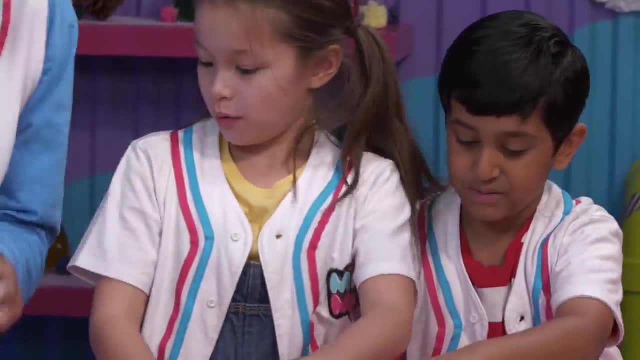 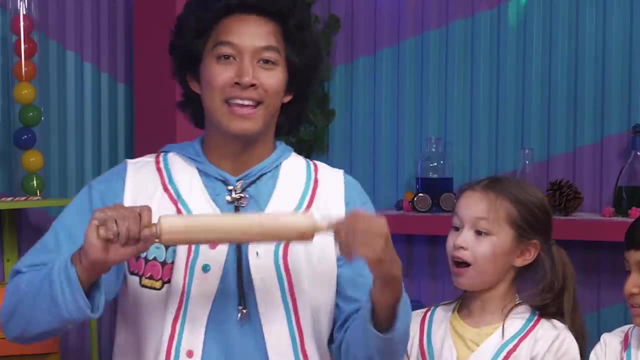 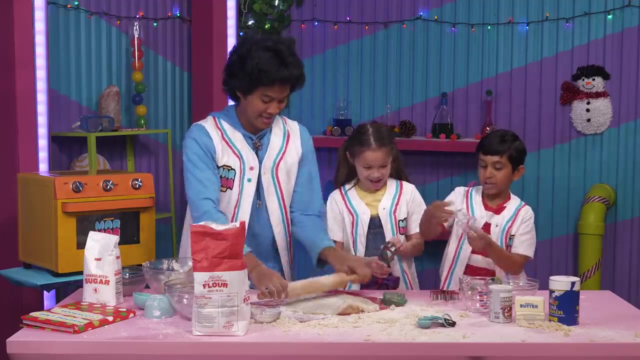 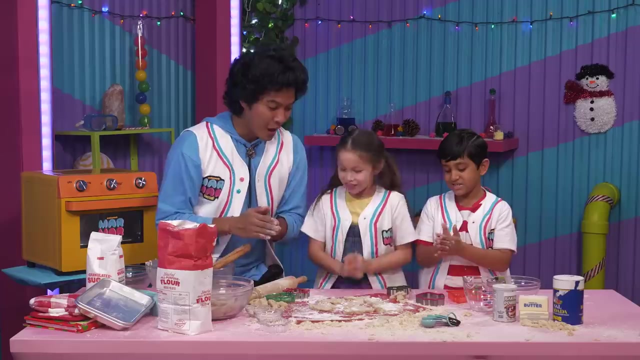 Oh my God, Oh, Ew, Oh, Ew, Ew, Ew, Ew, Ew. pen and roll it out and cut it out, these cookie cutters. okay, it's time to put them on trays and bake for 12 minutes. go ahead and place them on the tray and. 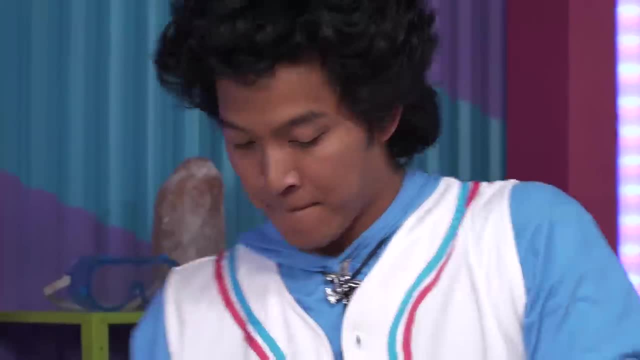 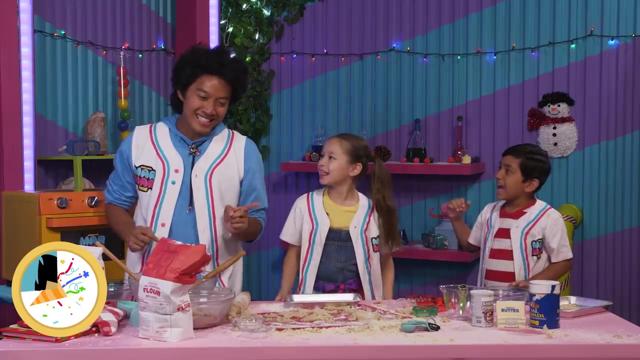 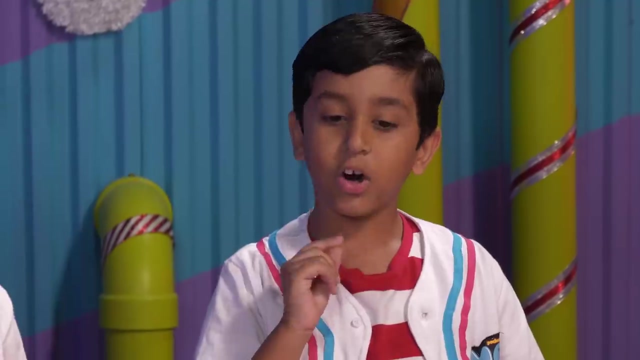 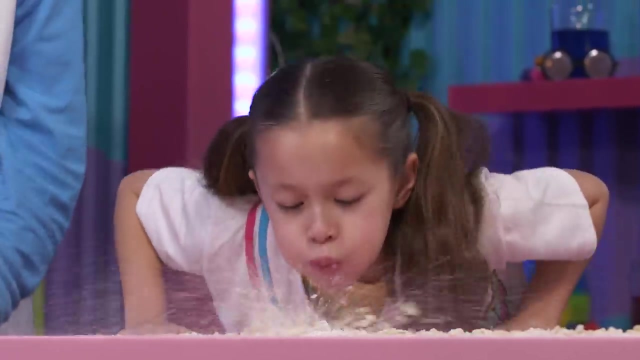 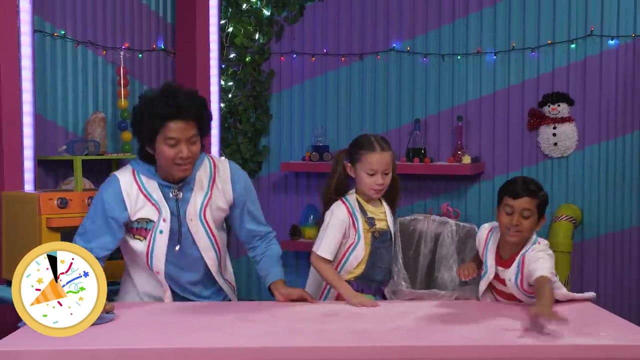 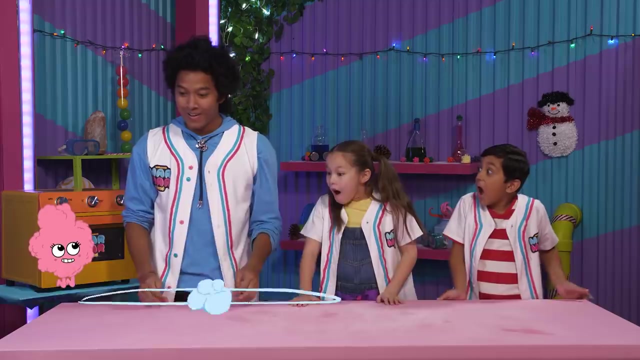 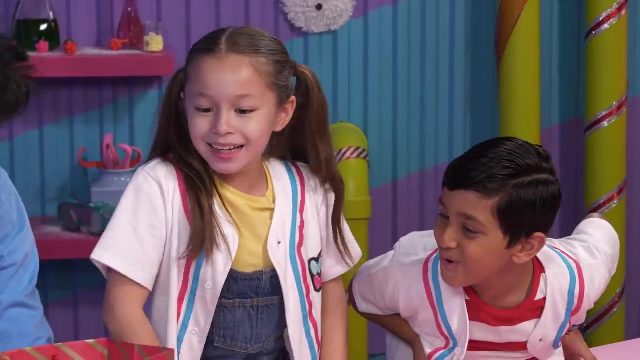 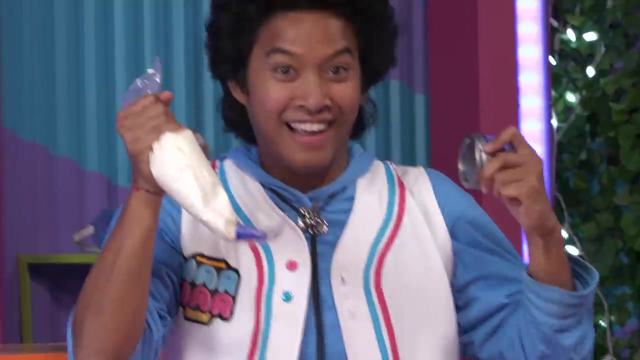 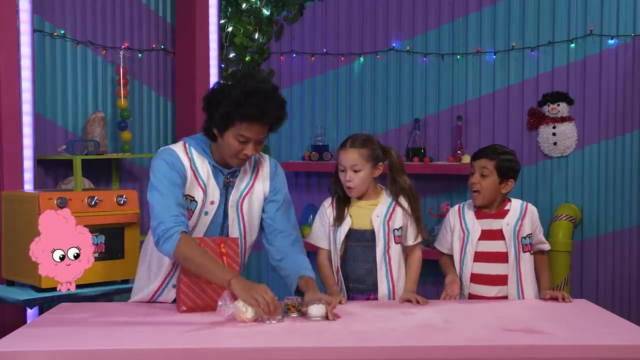 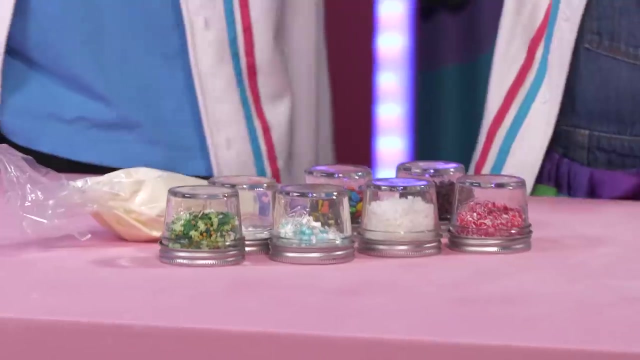 I'll handle the other part, okay, okay, not exactly. the last step is to clean up. always remember to clean up after yourself, after baking or cooking, always. all right, let's clean up. we did it and just in time, now I have the surprise ingredients. a good holiday cookie without beautiful cookie decorations? let's decorate. 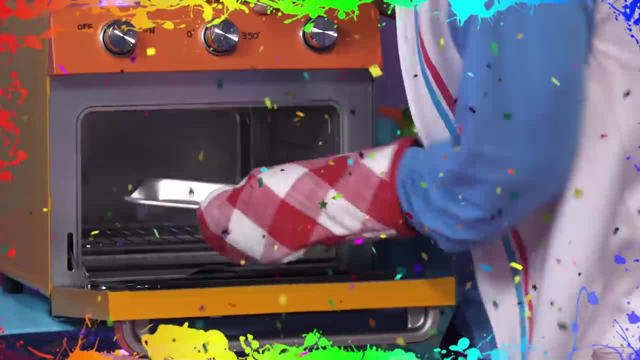 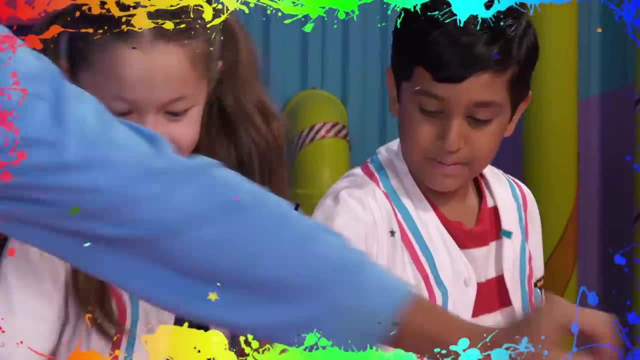 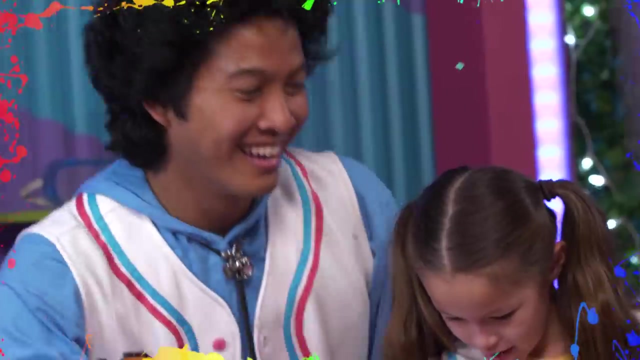 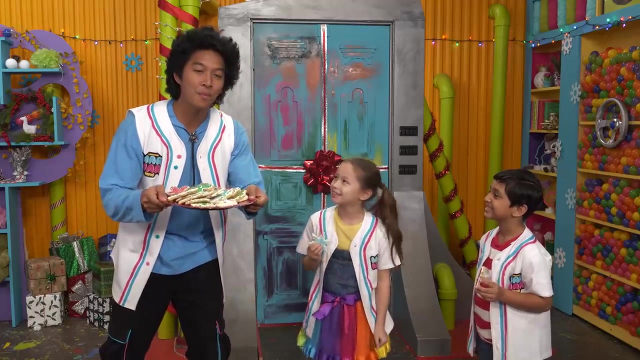 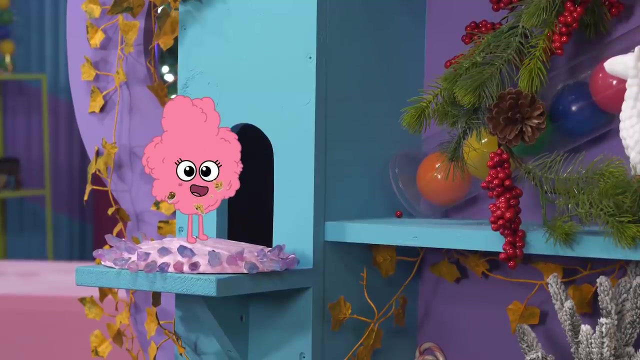 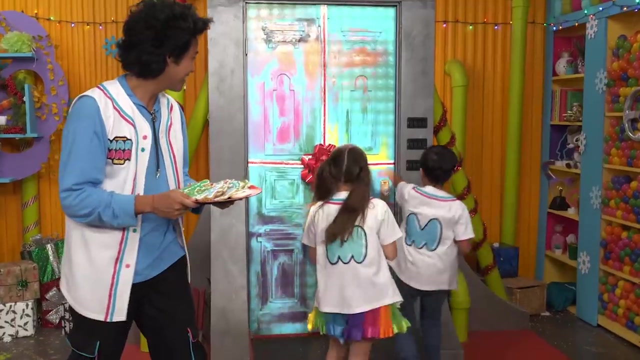 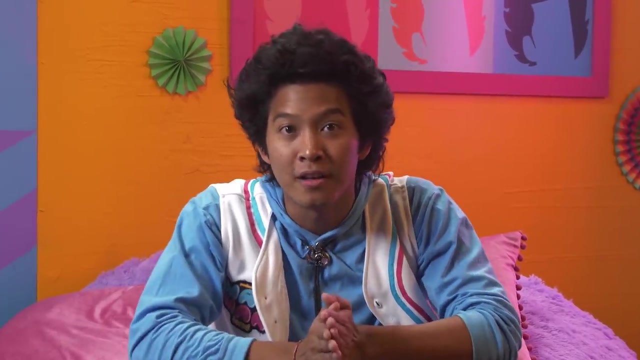 cookie party. these are the best holiday cookies ever. I want to make them with cookies with my family. thank you both for helping me learn how to bake and thank you to cloudy the delicious cookies. bye, cloudy, bye, explorers. explorers, baking can be hard, but if you read a recipe carefully and ask for help, 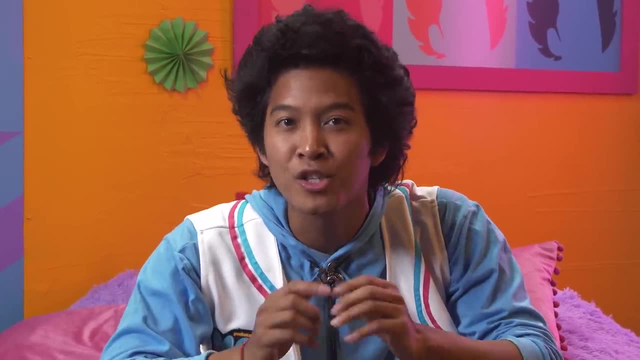 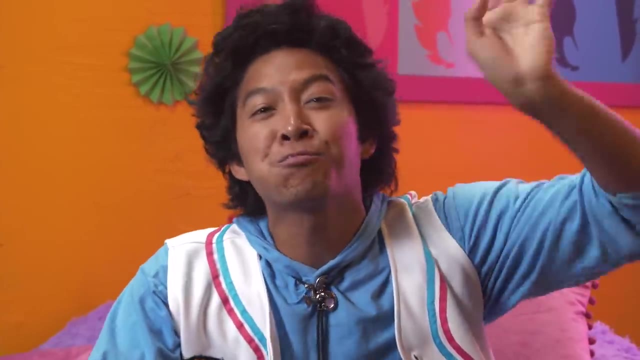 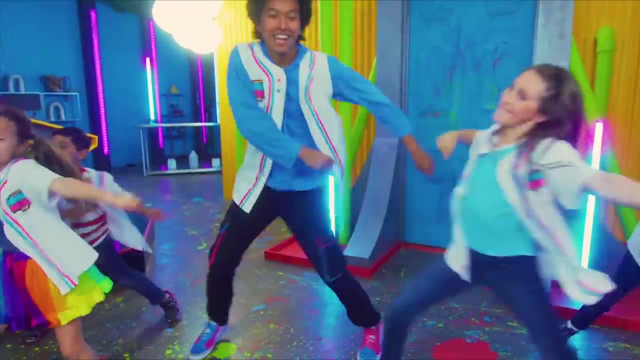 whenever you need it, you can be the best chef on the block, and once you learn how to bake and cook, You can make the things you love all by yourself. I'll see you next time. Bye Fours. This is good. You want to make the world a better place. Share, smile, illuminate, don't hate. Never hesitate to. 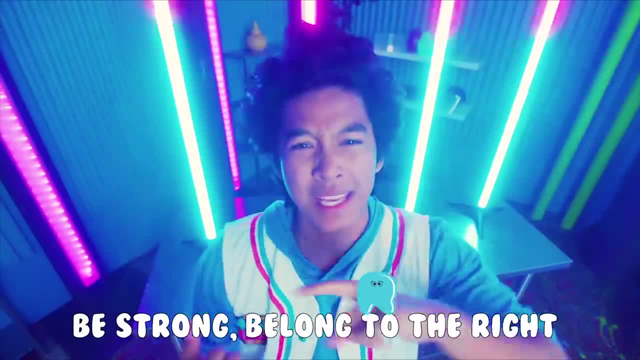 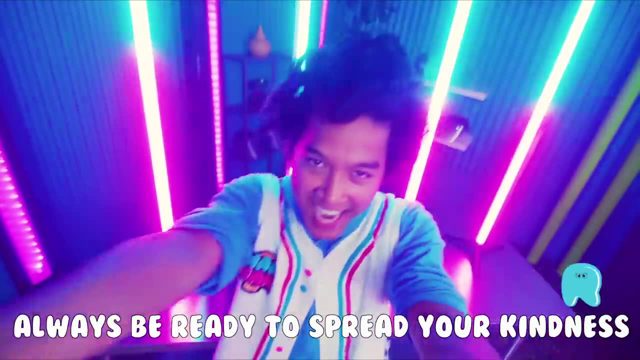 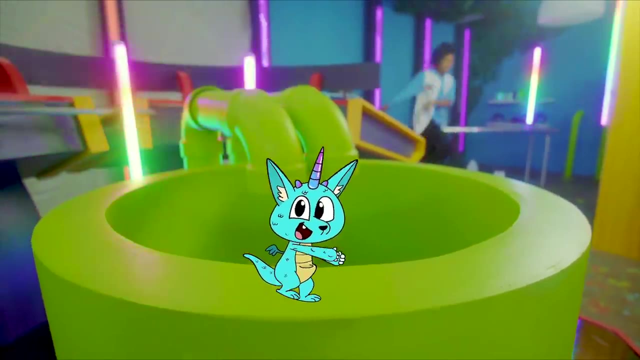 pour peace and love into every day. Be strong, belong to the right, not wrong. Look up, look down, look all around till the truth be found, And always be ready to spread your kindness like confetti. Come on, spell it with me, F-A-R, Uh-huh, F-A-R, Let me hear you. L-A-N-D Marmarly.